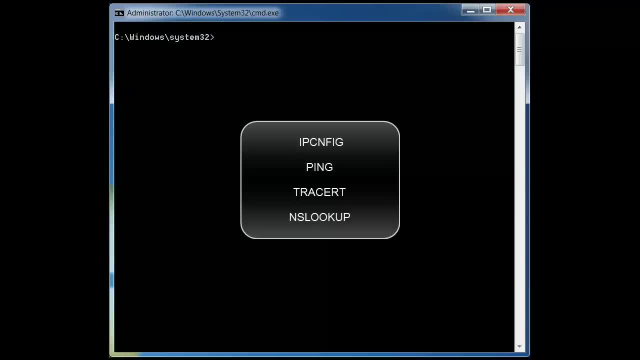 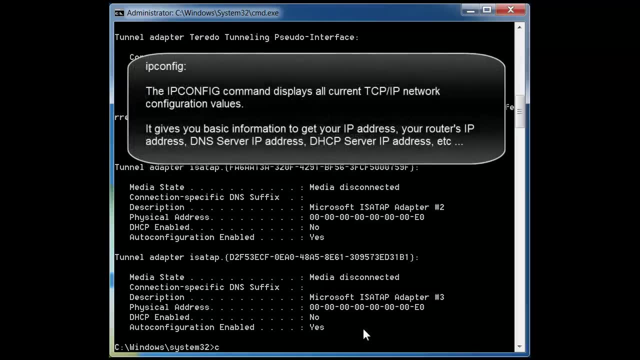 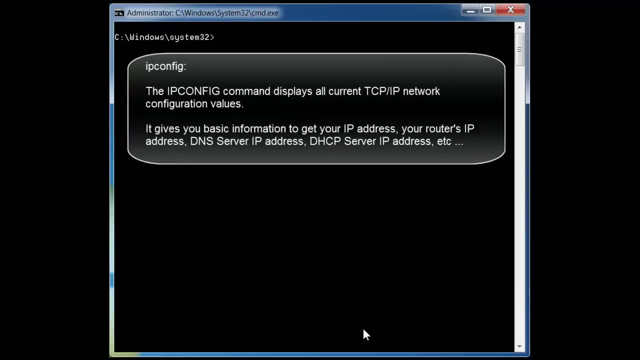 So let's start with ipconfig for now. Okay, so the first command that I want to go over is the ipconfig. The ipconfig command is a very common and very useful tool. It displays the current information about your network, So it will give you basic information, such as your IP address for the computer that you're stationed on. 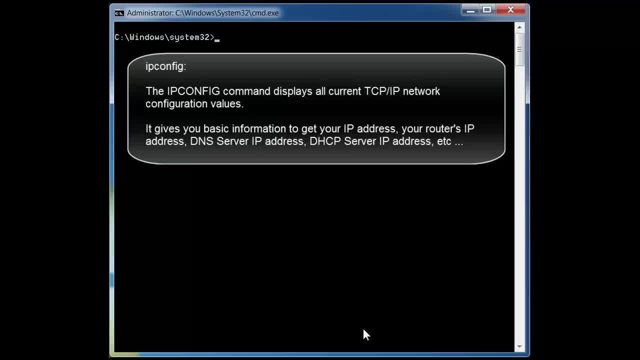 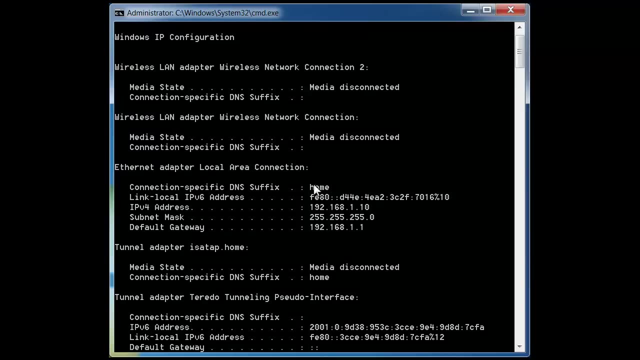 It will give you the IP address of your router. It will tell you where your DNS servers is, where your DHCP servers are. So let's type in the básicamente ipconfig command to start, And usually your local area connection is called the Ethernet Adapter local area connection. 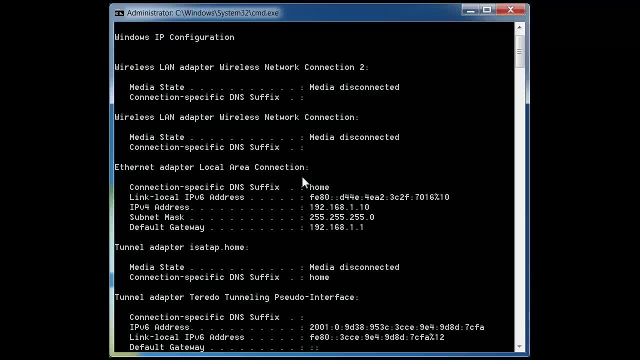 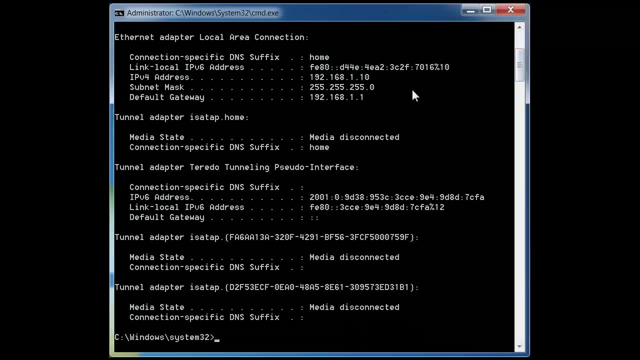 So this is the connection where you plug in your network cable. The RJ45 network cable connects to the jack behind your computer and this is the information pertaining to that plug-in connection. anyway, you can get your ip address on this screen, which is 192.168.1.10. it's also. 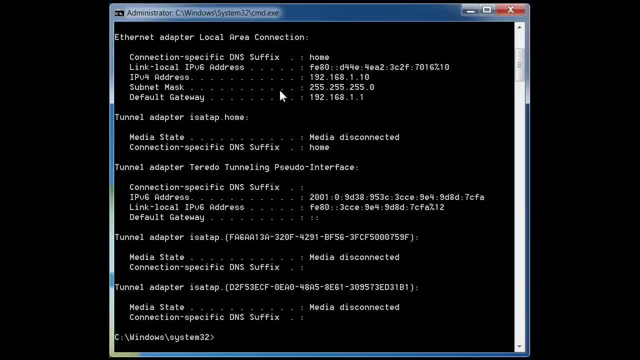 called the ipv4 address. you can get your subnet mask right here and you can get your default gateway address here. the default gateway is your router, so now i know the ip address for my router by looking at this screen. um, as you can see, you don't get much information about your local area. 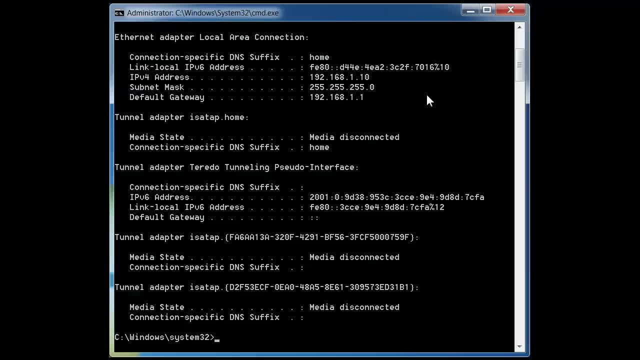 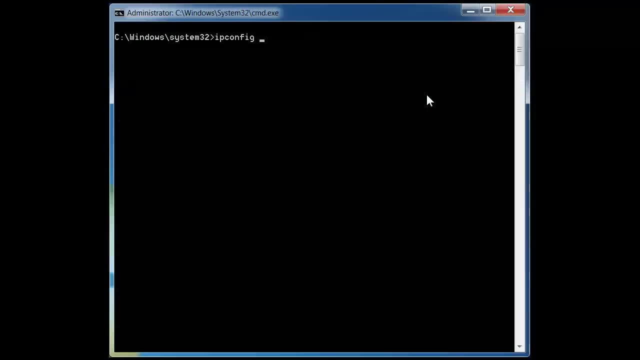 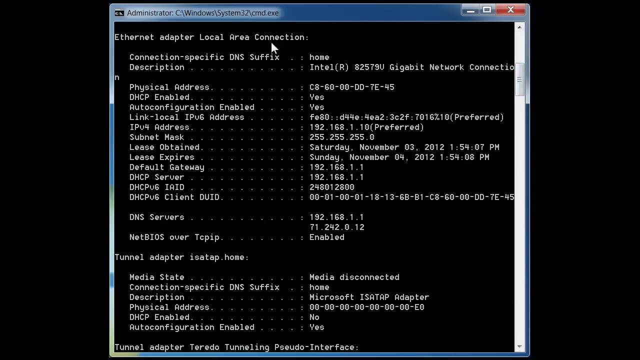 connection here. so what i'll do is i'll clear the screen. type in cls to clear the screen and type in ipconfig slash- all to get more in-depth information about your local area connection. press enter and let's go back up to the ethernet adapter local area connection. this time, as you can see, there's much more information present. 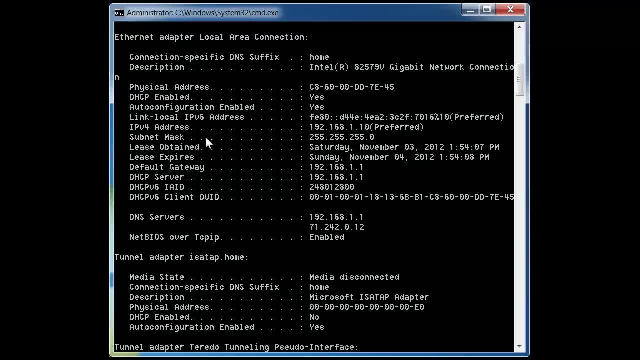 the ip address is still here, the subnet mask is still here, the router address is still here, but this time you can also see where is your dhcp server. in my case, as you can tell, the ip address is the same as the router address. that means that my dhcp server is currently reciting. 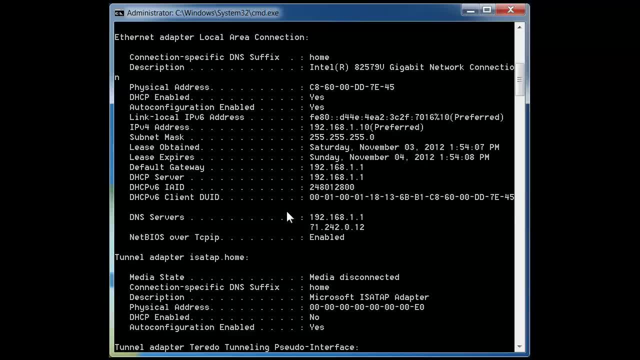 on the router and then your dns server. my dns server is also 192.168.1.1. it's the same as my router address. that means my dns server is also on my router. so you can see how this tool is helpful in troubleshooting and information gathering. information gathering is: 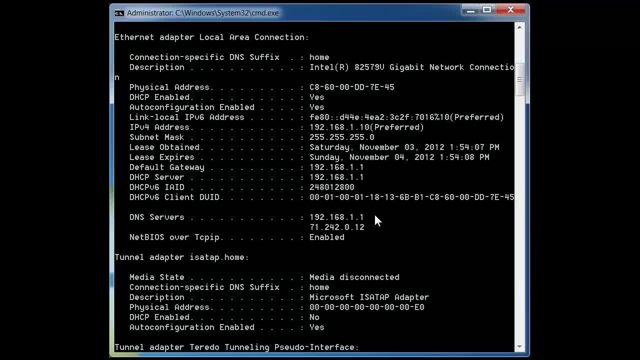 a part of troubleshooting. so, um, you know, when it comes to networks, the dns, dhcp, the default gateway, the subnet mask, these are all important keywords and you can get the information about these guys right here. so if you're trying to troubleshoot the dns server, you can beforehand type in the ipconfig command and find where the dns server is. so in my case it's. 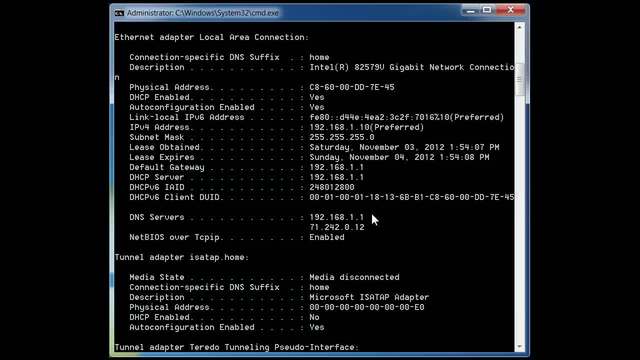 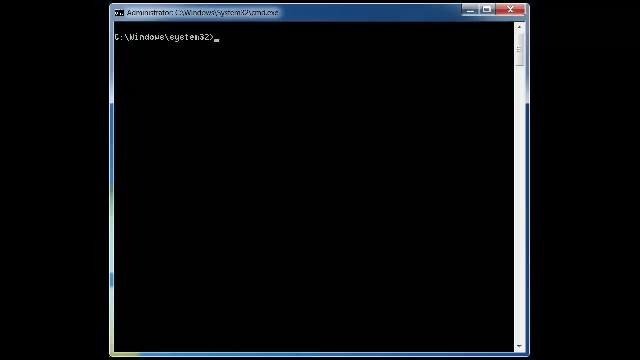 the router. so i would go to the router settings to tweak the dns server. okay, so let's, uh, let's move on to the next command. this is all i want you to know about the ipconfig command. so clear the screen and let's get on. okay, so one of the commands you'll be using a lot for. 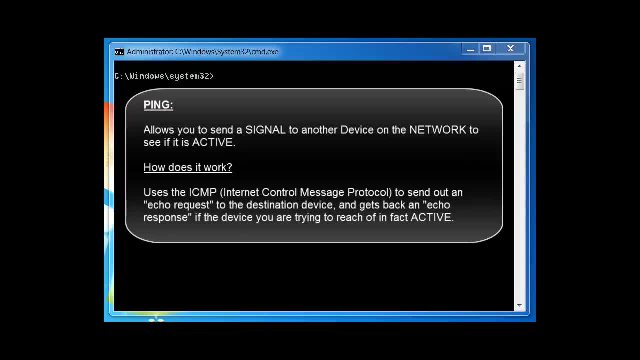 network troubleshooting is the ping command. ping command allows you to send a signal to another device and if that device is active, it will send a response back to the sender. now for those of you who are interested in the details how of how this works, the the ping command is a subset of the icmp. 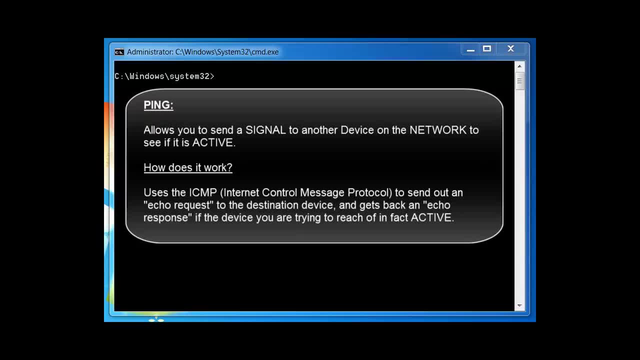 internet control message protocol and it uses what is called an echo request. so when you ping a device, you send out an echo request, and if the device you pinged is active or online, you get an echo response. so already you can tell why this is a good command to troubleshoot. 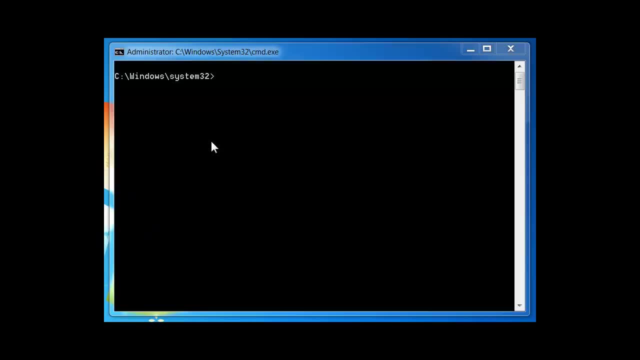 so, for example, if your router is down and you try to ping it and you get no response, then you know that the router is what is giving you problems. so let's, uh, let's run this command a couple times and see what kind of results we get. so let us let us uh ping my router. 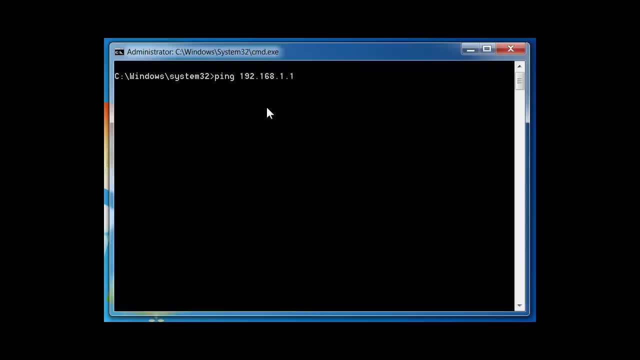 ping 192.168.1.1, press enter and let we will analyze the uh, the printout here that we got. so what happens is we send out four packets to the destination and the destination responds back with the same four packets. so you can see here one, two, three, four. so this is a reply from 192 168, one and one that is my router. 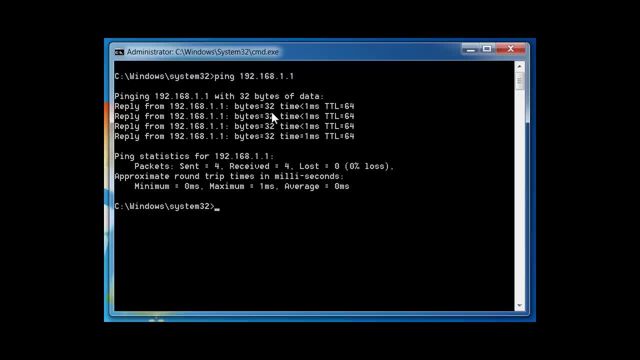 we sent out 32 bytes of data and we got back 32 bytes of data and we got it back in less than one milliseconds. down here you get a summary. so it says: packets sent, four, packets received, four packets lost, zero. so that means this is a stable connection. 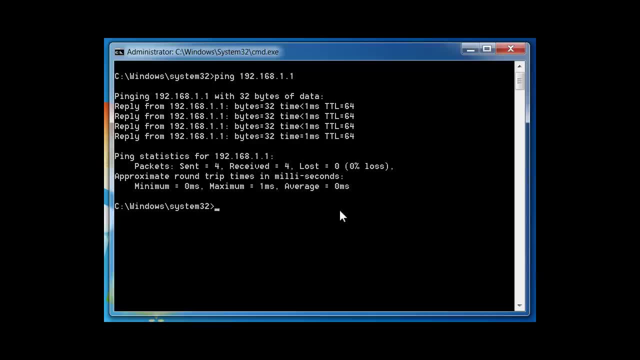 and then there's another- some statistics here. that is not important. so this is how the ping command works: it sends out an echo request using data packets of of minuscule size, and then you get a response and you know that the other device is actually alive. so let us ping um. 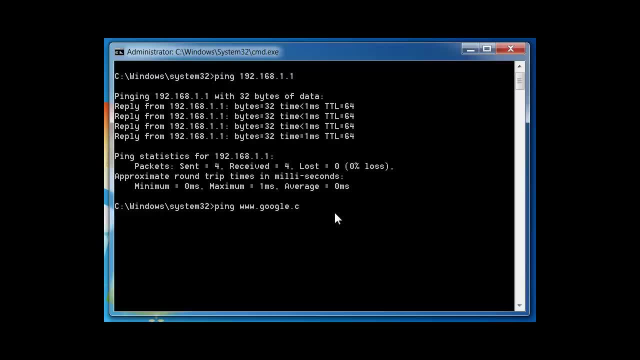 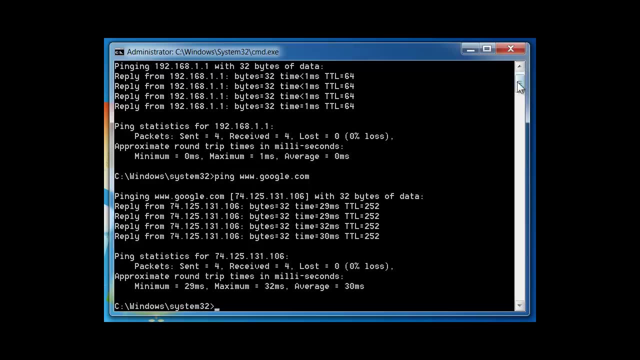 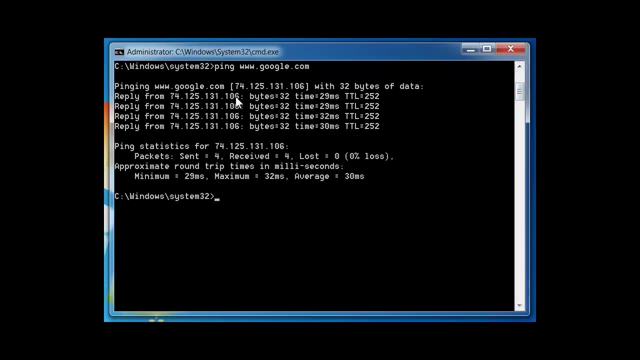 google, wwwgooglecom and see what happens. so we got a similar printout- let me just bring this to the top- and, as you can see, this is the ip address of google and that is where we got the response from. as usual, we sent out 32 bytes of data but, as you can see, because google is 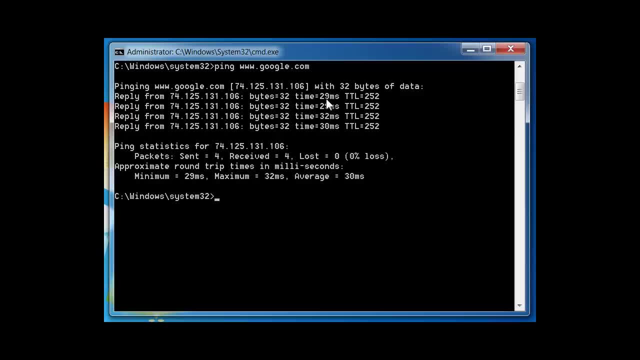 far, far, far away and not in my basement. um, it took 29 milliseconds to send uh to get a response from google and uh, if you look down here again, statistics are packets of data, strongly presented or a little bit. see more prices here instead of less than a hundred plus dollars. uh, so let's give. 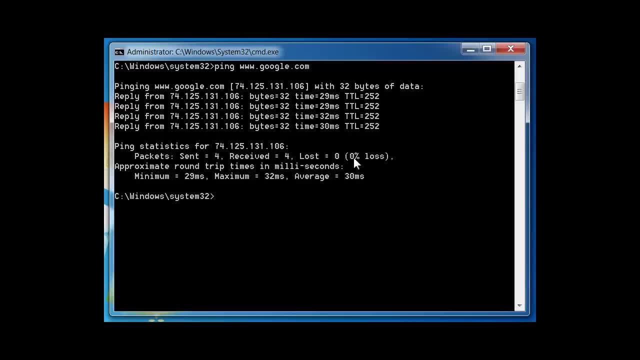 Our packets were sent, four received, four lost, zero, So the connection was stable. Finally, let's ping a device that doesn't exist. This is going to yield the same kind of results if a device wasn't actually working. So if your router was down and you pinged your router but you were not going to get a response from it. 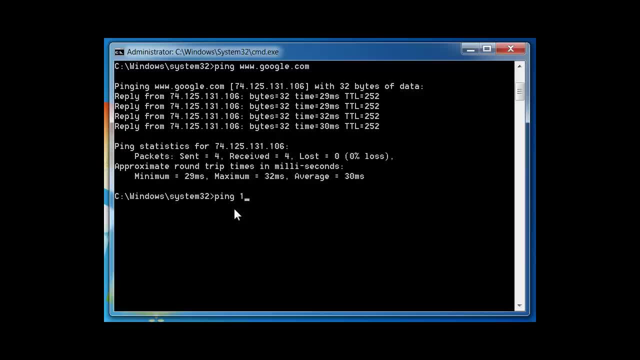 So let's see ping: 192.168.2.200.. Press enter. So we're pinging it right now And the request was timed out because that device does not exist. As you can see, the ping command is retrying. 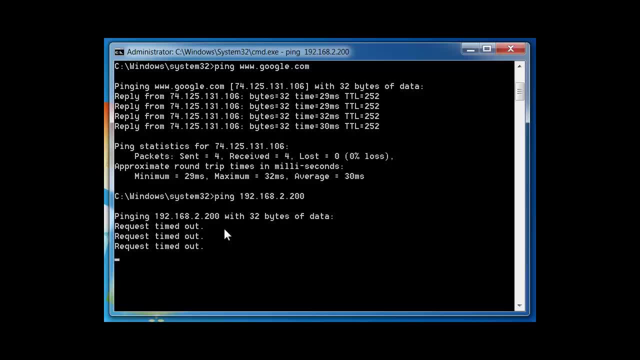 It's going to retry four times. The first packet didn't go through, Second packet didn't go through, The third packet And the fourth packet did not go through And, as you can see at the summary packets, sent four, received zero and lost four. 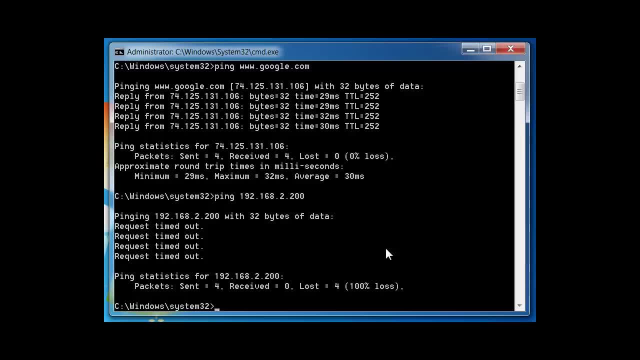 So it was 100% lost. The signal does not exist. So if you ping the device, you get no response and you lose all the packets. That means the system you're trying to reach is not connected to networks- having network problems. 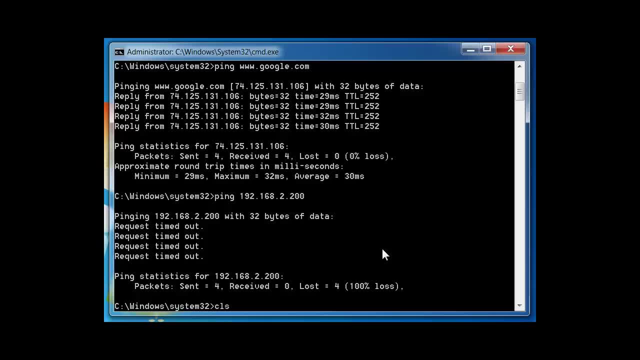 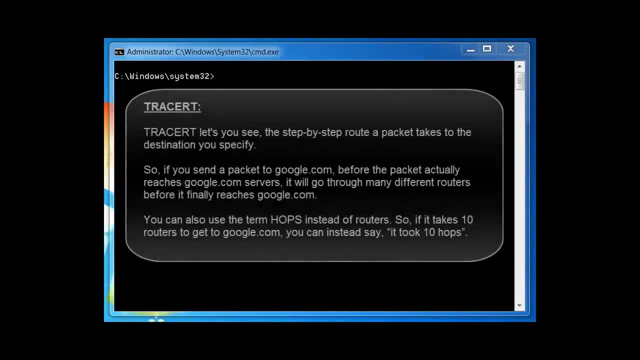 And this brings us to the end. So we're done with the ping command. Let's clear the screen and move on to the next command. So the next command is the traceRT command. So what the traceRT command does is it lets you see, step by step, a route a packet takes to the destination that you specify. 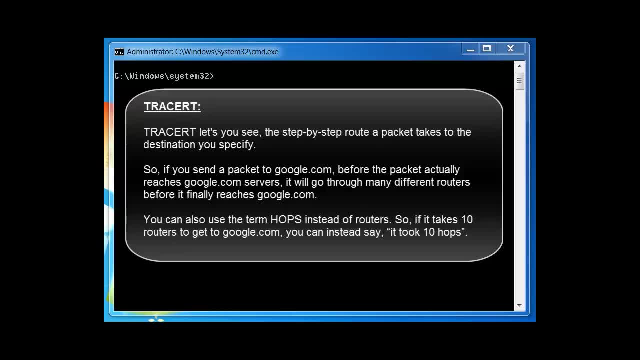 So if you send a packet to googlecom, before the packet actually reaches googlecom goes through a couple of routers to reach the destination, so it'll go to your router, then it will go to Verizon or Comcast router and from there it's going to go to all kinds of different routers before it reaches Google servers. 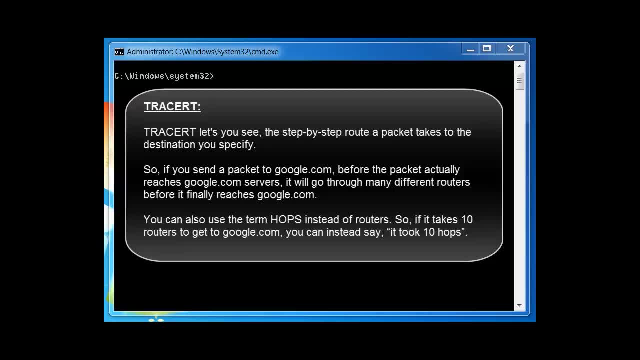 so you can also use the term hops instead of routers. so if it takes 10 routers to get to googlecom, you can instead say it took 10 hops. so how do you do, how to use this, this command for troubleshooting? let's actually run the command and see what kind of results we get. so I'm going to 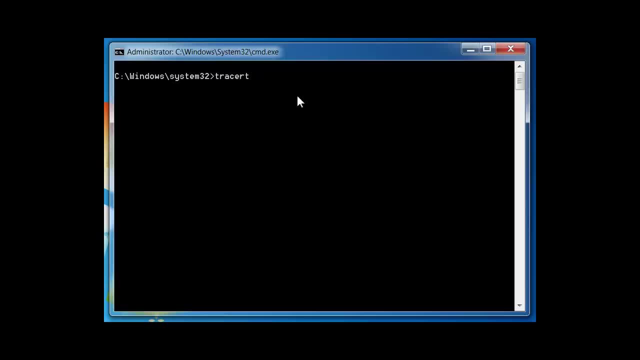 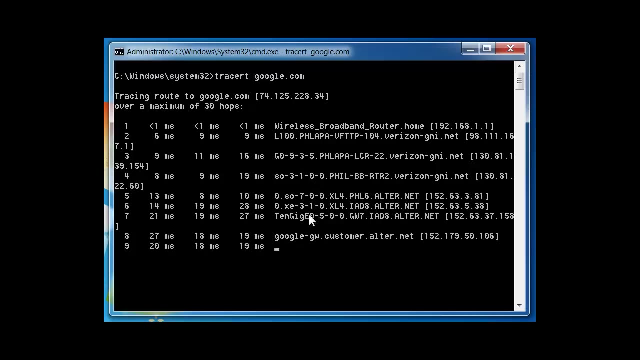 run the trace RT command and I'm gonna trace googlecom. okay, so, as you can see, we're getting a list of each of the routers that we are hitting as we are closing in on googlecom and up here, it will tell you what you're tracing and it'll give you the IP. 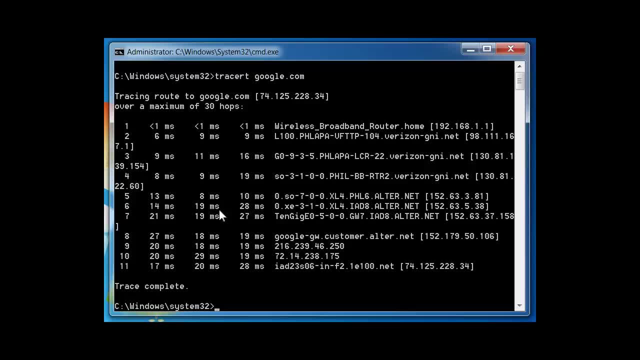 address for our Google. okay, so the trace is complete. let's see, we have one, two, three, four, five, six, seven, eight, nine, ten, eleven. we went through eleven hops, eleven routers before we actually reached googlecom. now, if you look up up top here, the first router that we actually hit was my own router. I can tell by the 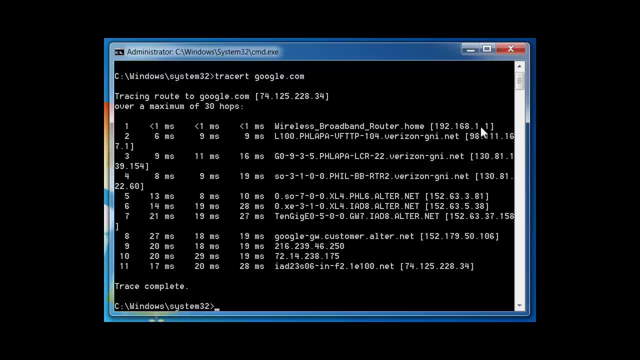 IP address right here: one, nine, two, one, six, eight, dot one dot one, and it's the wireless broadband router dot home. the next one, because I have my service through Verizon, was Verizon's router, so it clearly goes step by step through all the hops and then, after eleven hops, we 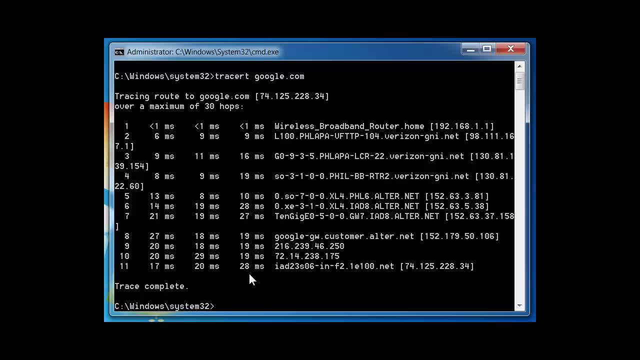 were at googlecom. what, what? what is the significance of this? let's say, your home network was perfectly fine, but there was a problem with the Verizon routers. you can run the trace RT command and if, if there's any problems here, it will actually tell you what the 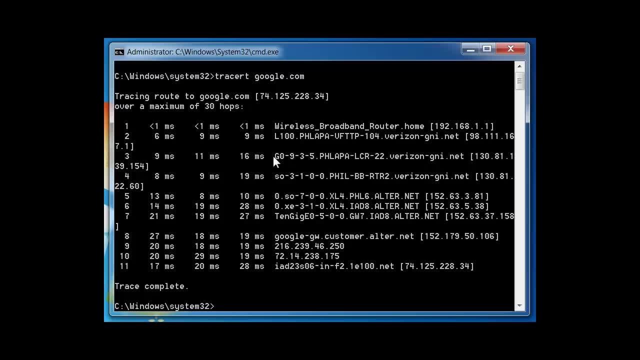 problem is it could say things like request timed out, destination destination unreachable, or it could also say that in so 16 milliseconds it could be saying like 5,000 milliseconds, just to give an example, and I don't think you'll ever see that. but so if the request times out, that means the 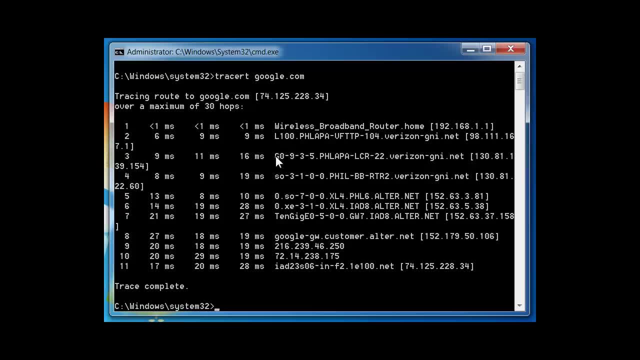 problem lies with one of the routers that has to do with Verizon, and then you can call Verizon and you can tell them: hey, you guys are having a problem because I know that my router works because I ran the trace RT command. so this is the idea behind the trace RT command. as far as troubleshooting goes, 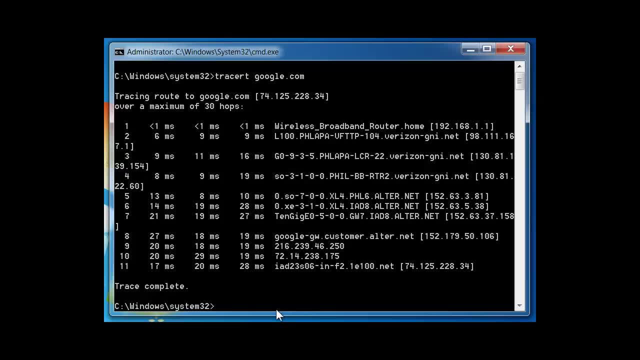 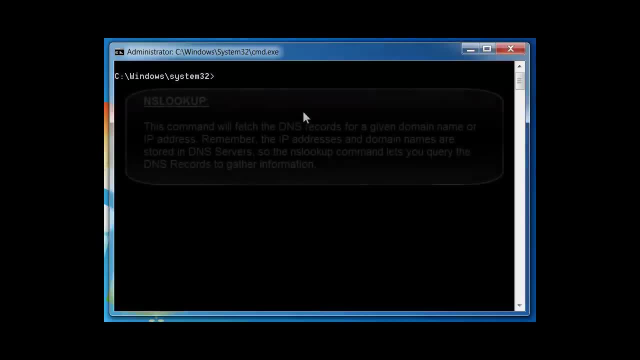 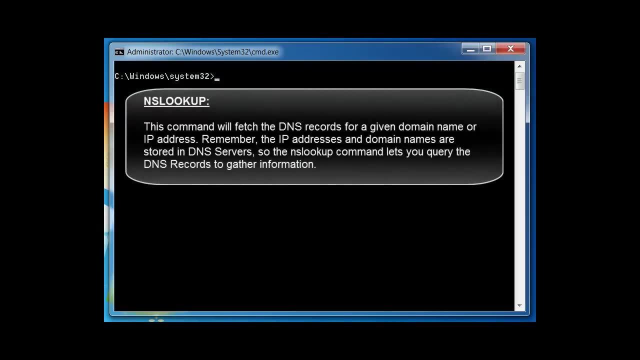 okay, so that brings us to the end of this command. let's clear the screen and move on to the final command. okay, so the final command I want to talk about is the NS lookup command. this command will fetch the DNS records for a given domain name or an IP address. 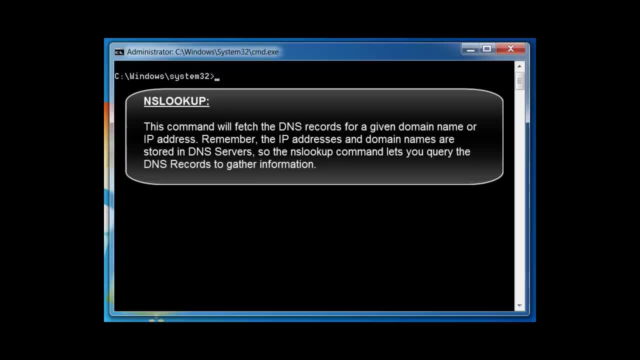 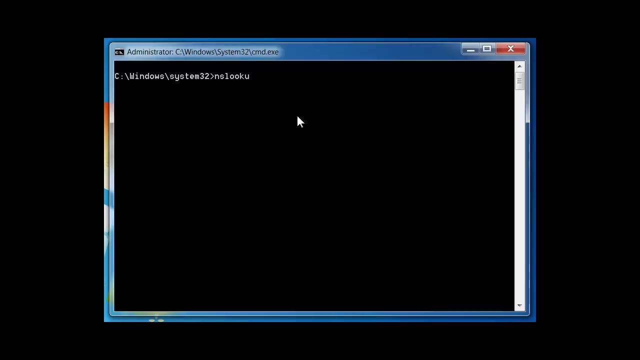 remember, the IP addresses and domain names are stored in DNS servers. so the NS lookup command lets you query the DNS records to gather information. so let's say I wanted to know the IP address of googlecom. I could simply type in NS lookup and and type in googlecom. 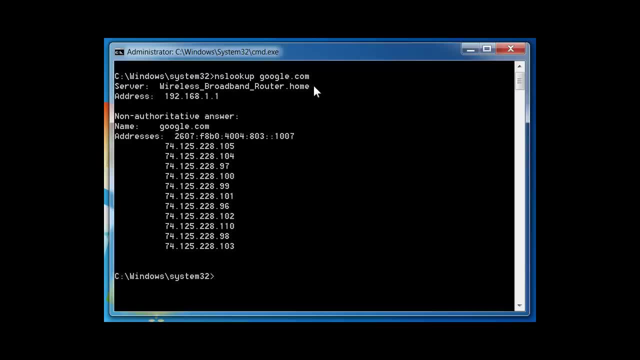 and press enter and what? let's analyze this printout. so the the first two lines here show you which DNS server was used to get these results. my DNS server happens to reside on myartsexe format or some sort of SNAP server, for Thats Bliss. その DNS. Well, if you see my Keeler server, here the DNS server is implied as the dot Felipe. and then? so this IN百切。I don't know. so the first two lines here show you which DNS server was used to get these results. my DNS server happens to reside on my brethren length. 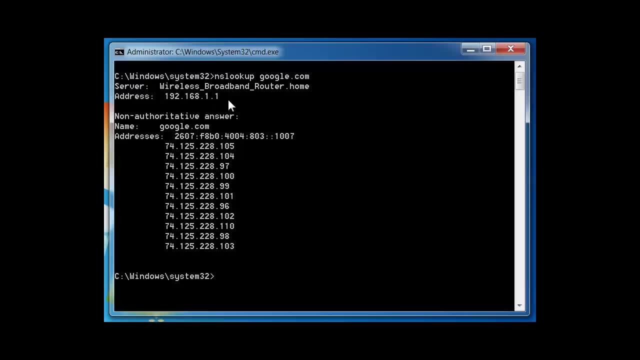 router. as you can see, 192.168.1.1 is my router, so that is also my dns server, and the answer that we got was this: all these ip addresses here are google's ip addresses. now, google is a huge website. obviously it's not going to have one single ip address and obviously the ip addresses 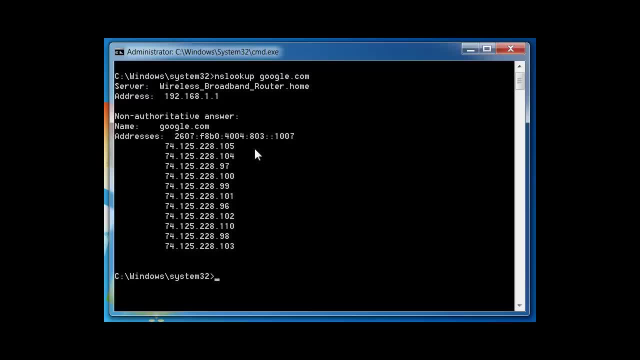 will change from time to time, but if you type in any of these ip addresses in your browser, it will take you to googlecom. uh, so this is the uh basic idea behind the ns lookup command. okay, so this brings us to the end of this video and, uh, if you guys liked the video, just click. 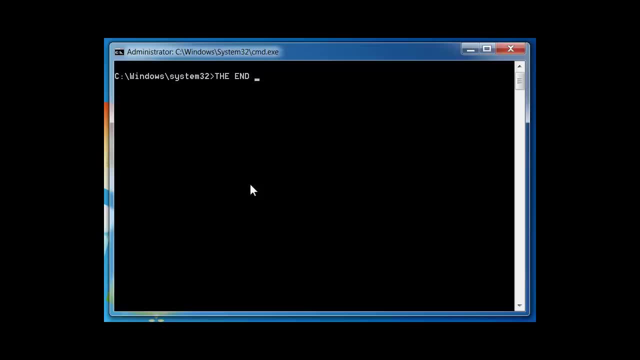 the like button and, if you like my videos, subscribe to my channel, because i will be updating more and more videos of this sort and, uh, thank you for watching. have a good day, guys. 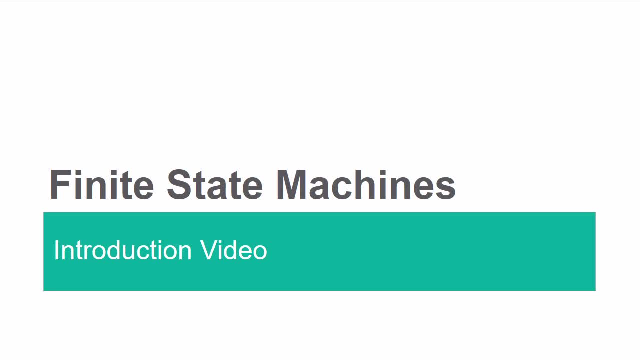 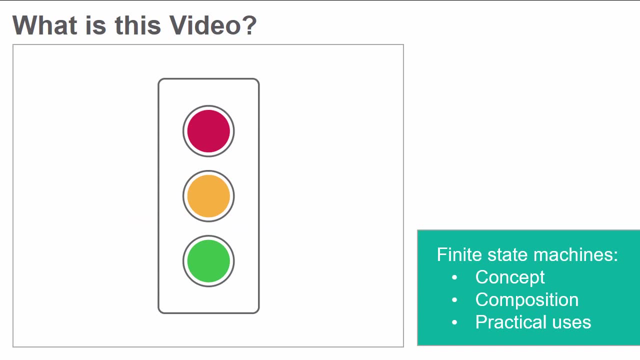 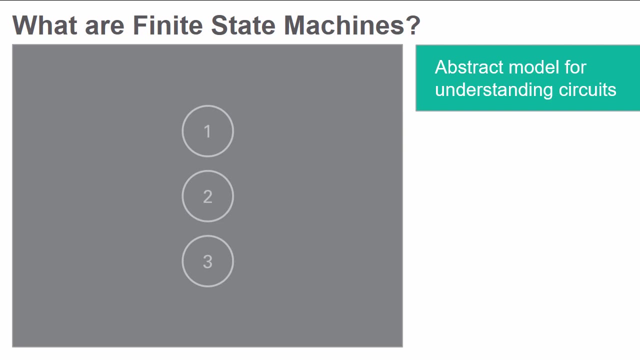 Introduction to Lab 12- Finite State Machines. In this video we'll discuss the concept of finite state machines, their composition and their various practical uses. A finite state machine is an abstract model used to understand certain types of circuits. In all finite state machines there are a discrete number of states in which the system can exist. 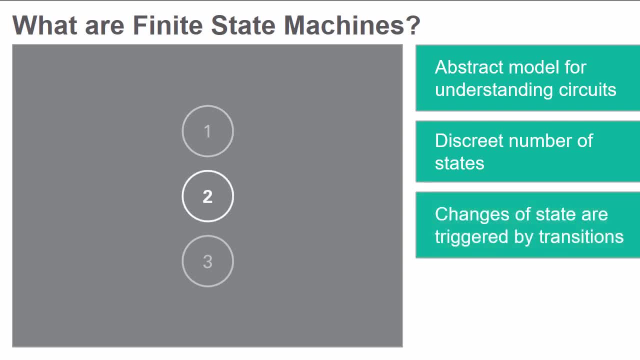 Changes of state are triggered by particular events, known as transitions. The machine can only exist in one state at any given time, known as the current state. This concept, unlike the others in the digital electronics course, is abstract and therefore there is no specific chip or combination of logic gates that form the basis of all finite state machines. 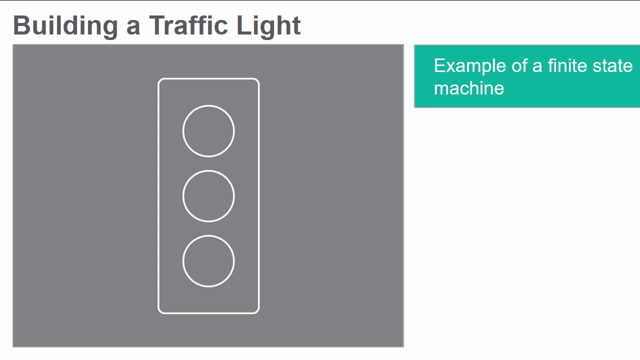 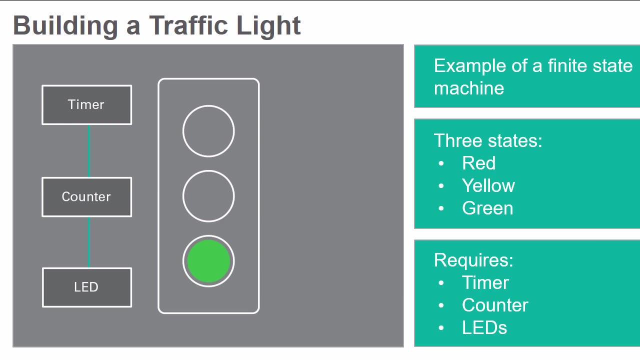 A practical example of a finite state machine is a traffic light signal. The three possible states for this machine are red, yellow and green. This can be simulated in PLD design using a timer, a counter and LEDs. The counter and timer are used to determine how long each state exists. 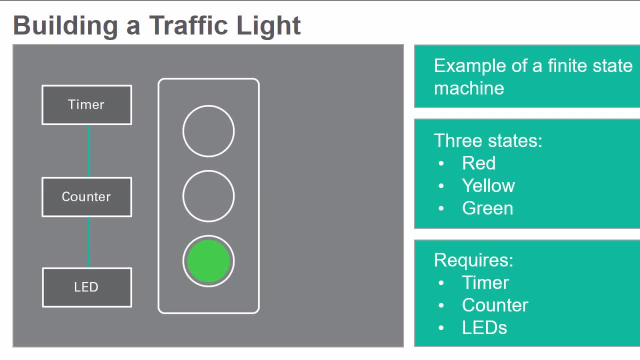 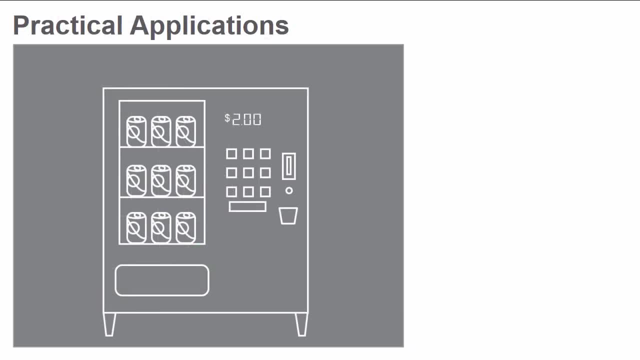 and when the transition between states occurs. Because of the circuit's complexity, it will contain a main circuit as well as additional sub-circuits. Finite state machines have a variety of other uses as well. They are used in vending machines to dispense product when the appropriate amount of money is deposited. 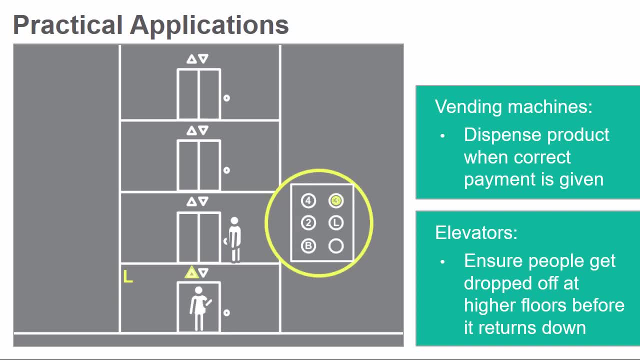 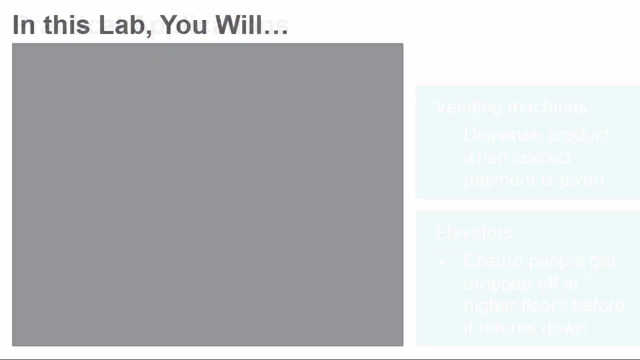 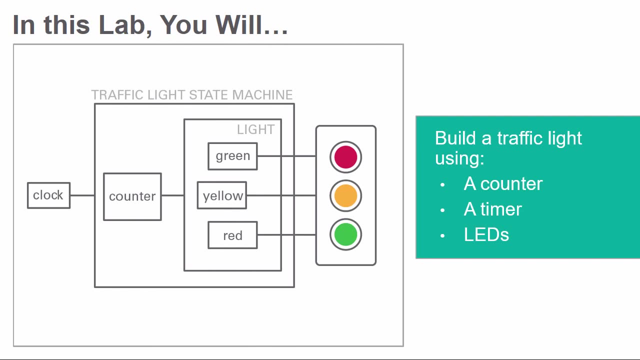 They are also used in elevators to ensure people are dropped off on the top floors before the elevator comes back down. In this lab, you will be building and testing your own finite state machine: a traffic light in PLD. This design requires a counter, a timer and LEDs.